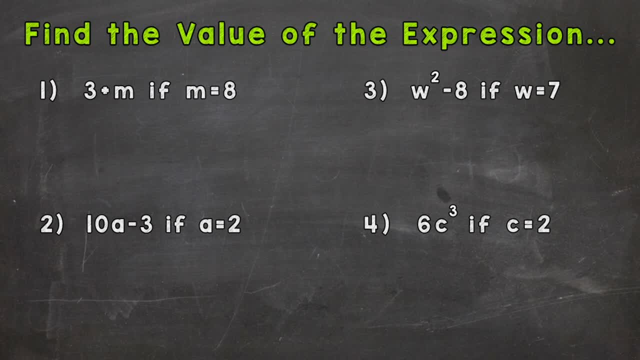 m equals 8.. So we would read this: find the value of the expression 3 plus m if m equals 8.. So that m, within our expression, is our variable, our missing piece. Well, we are given what the value, or how much that m is worth, right here, m equals 8.. So, in order to solve, we need to plug that 8 in. 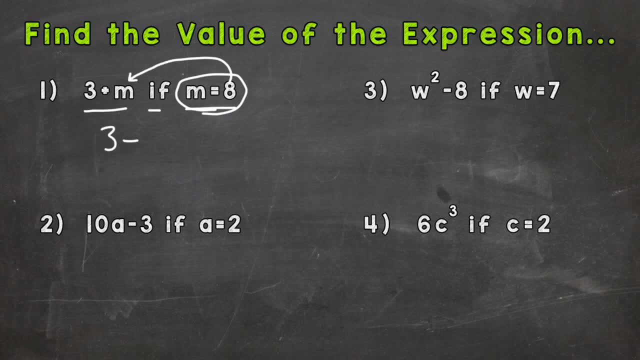 for m. So we would have 3 plus 8, and now we're able to solve and that will give us the answer or value of the expression, and 3 plus 8 equals 11.. So that's our value or answer to number one. 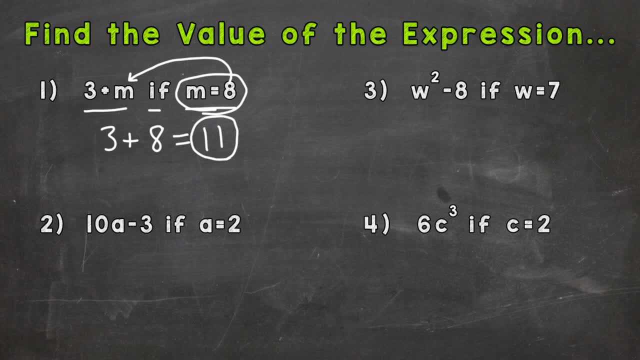 Number two: we have 10a minus 3.. So find the value of the expression 10a minus 3 if m equals m. So we would have 3 plus 8, and now we're able to solve and that will give us the. 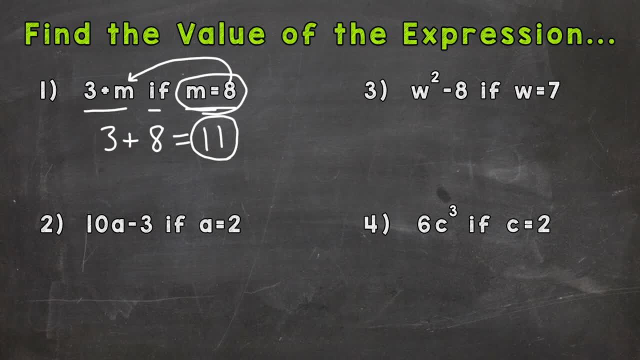 if a equals two. So right here, where we have a number right next to a letter, whenever you see that, that means multiplication. So that means 10 times a or 10 times the value of a. So let's rewrite our problem: with two plugged in for a, 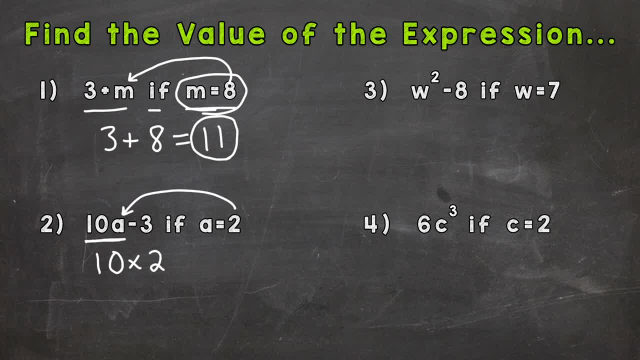 So 10 times two minus three, And now we're able to solve- So it's just order of operations- which multiplication comes before subtraction. So 10 times two is 20.. Bring down our subtract three And we get the 20 minus three, which is 17.. 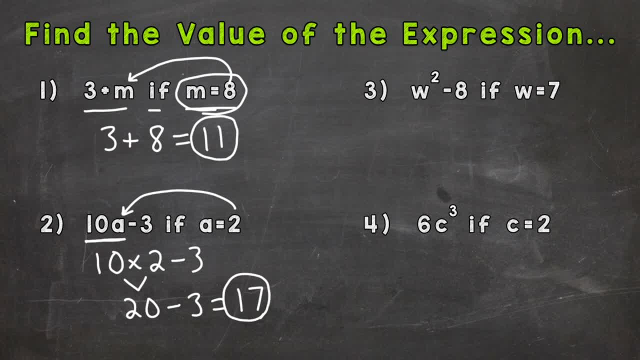 Number three: we have w squared minus eight. So find the value of the expression w squared minus eight if w equals seven. So again we need to plug in the value of our variable, which in this case it's a seven. So we have seven squared minus eight. 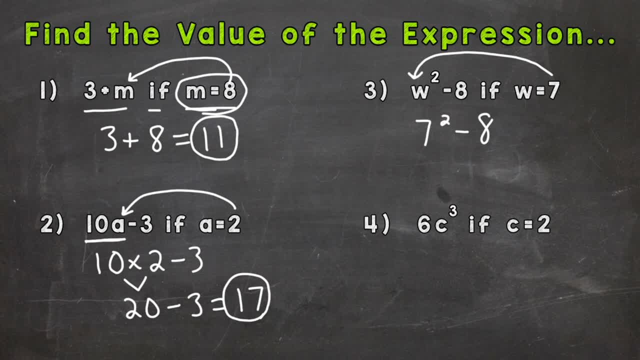 So now we're ready to solve. So order of operations. exponents comes before subtraction. Seven squared does not mean seven times two. Remember an exponent means to expand that seven out twice. It means to multiply. So it means seven times seven, which is 49..